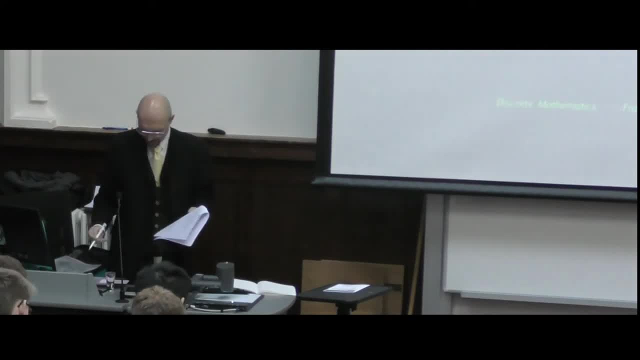 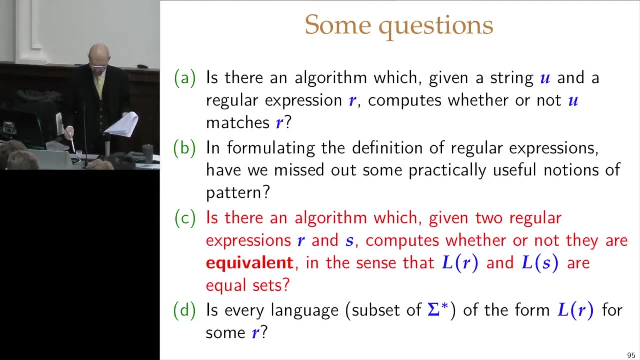 they are derived from the basic ones we originally introduced and therefore, if we look back at our list of the grand questions, this part b, in formulating the definition of regular expression, have we missed out some practically useful notions of pattern? well, we see that with the pretty basic, 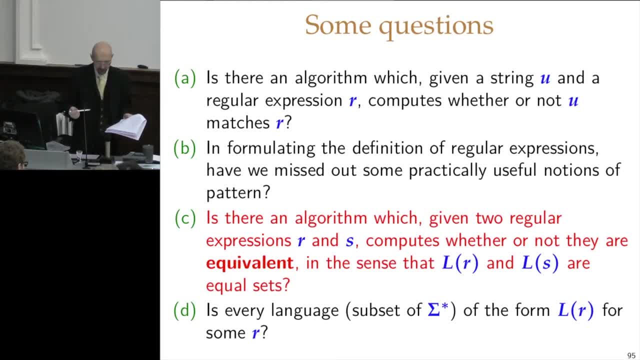 stuff that we originally had in our definition of regular expression. we can actually construct many other elaborate operators, Including not just the trivial ones, which are syntactic sugar, but some serious ones like complementation and intersection. We already had the union, so we now have basically all the set. 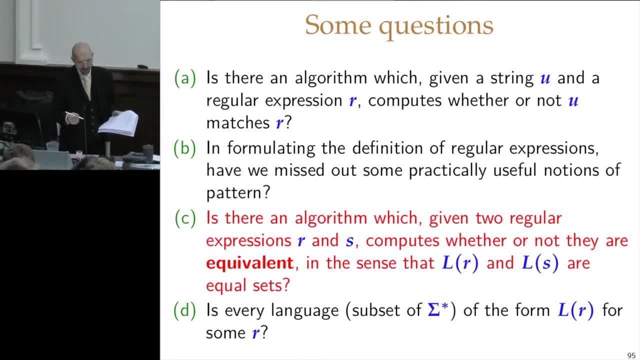 theoretical primitives as part of our regular expression arsenal. So this allows us to move on to another question: Is there an algorithm which, given to regular expressions r and s, computes whether or not they are equivalent in the sense that they recognize the same language? And this is something you might want to do. in practice, You are given two regular expressions. 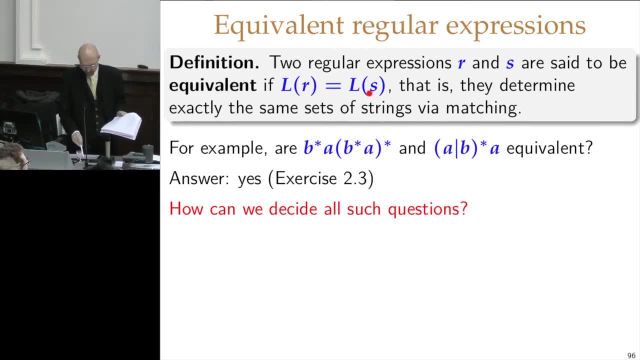 The definition is obvious: they are equivalent if the language the first recognizes is the same as the language the second recognizes, So the set of strings is the same in both cases. This regular expression: b star, a, b star, a star. what does this do? well, you can have as many bs as you like, including 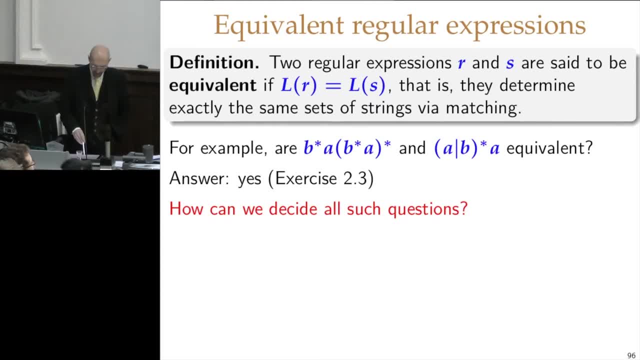 none, then you have to have an a. then you can have as many of these brackets as you like, including none. and if you have any of the brackets, you can have as many b's as you like and then one a. because you have a star in here. you might not have any a's but that a nobody's excusing it from having. 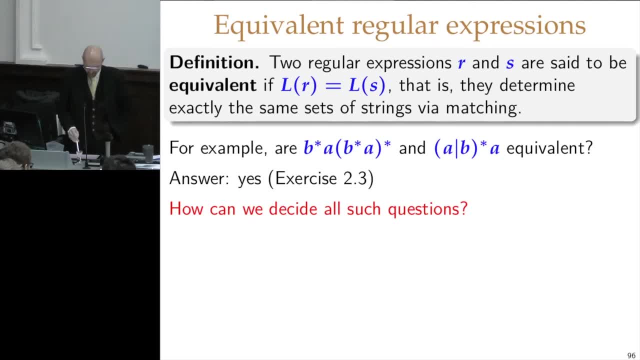 that one. so you have to have at least that A and the claim, or the claim or the question is: is this equivalent to A or B? star meaning any symbol including nothing, any sequence of the allowed symbols A and B, including the empty one followed by an A. you think these things are equivalent. who thinks they're? 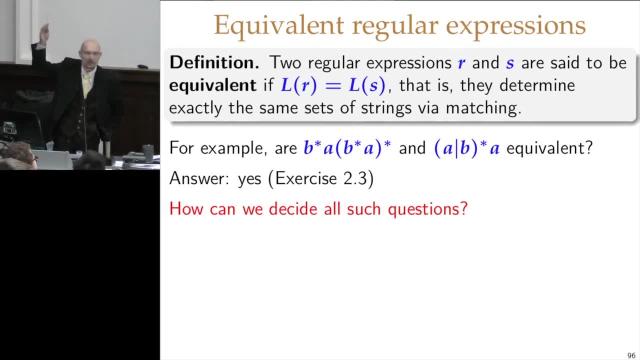 equivalent. who thinks they're not equivalent? almost no, okay, all right. well, let's see how there's an answer here. all right, you have to figure out when you answer exercise 2.3. how is it possible that here I have to have this A and then I must still have some B's. 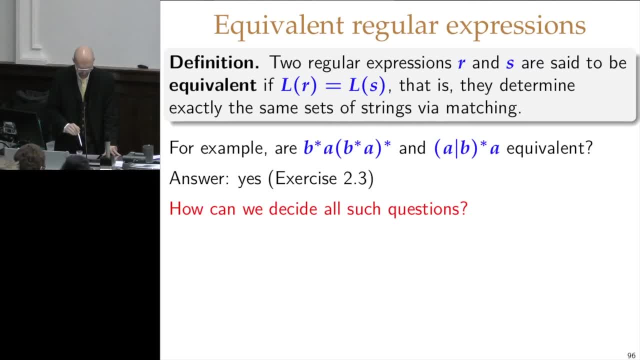 after that, coming from this parenthesis. but there's no way to have a B after this A over here. how's that possible? hint, it's possible because there's another A that's not there, and then there's another A that's not there and that's forced in here. anyway, do the exercise yourself and then we'll see. but 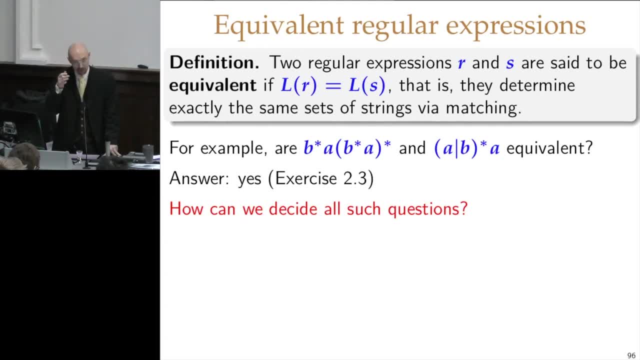 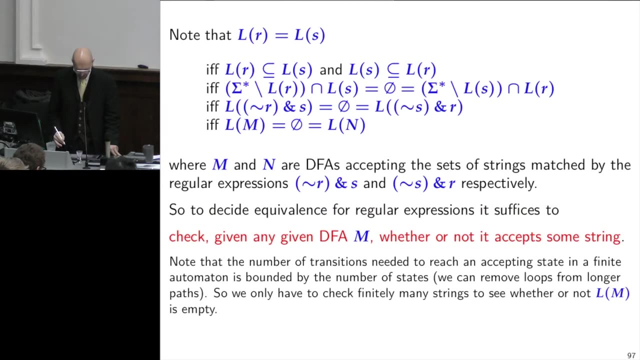 what we're going to see next is a general method, although not a practical one, to do in your head, a bit like the second part of Kleiner's theorem. it's a method that works systematically all the time, but it's not the easiest thing to actually answer the question on a piece of paper, and what we do is we use our 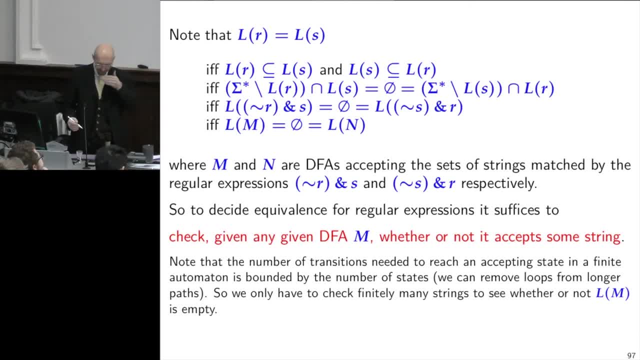 now full complement of self-theoretical operators to do the following reasoning. excuse me, the language of the strings recognized by regular expression R and the language of the strings recognized by regular expression S are both subsets of the universe of all the strings that can be made in Sigma star with characters in Sigma. all the strings I obtain are Sigma star. 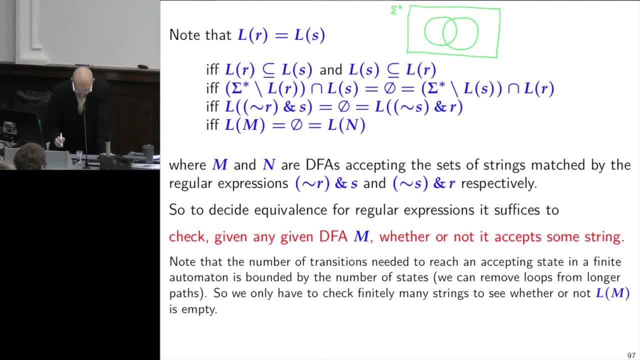 this is the rectangle, is Sigma star, and this is the strings recognized by regular expression R and the strings recognized by regular expression S. these two languages are the same if, and only if, this region is empty. and this region is also empty if it is true that this, these two things are. 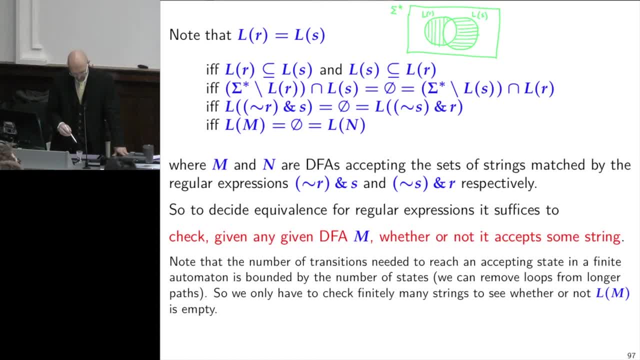 crossed out are empty, then these two sets are equal to each other and to their intersection. and this is equivalent to saying that the language recognized by R is included in the language recognized by S and, at the same time, the language recognized by S is included in the language recognized by R, and this again. 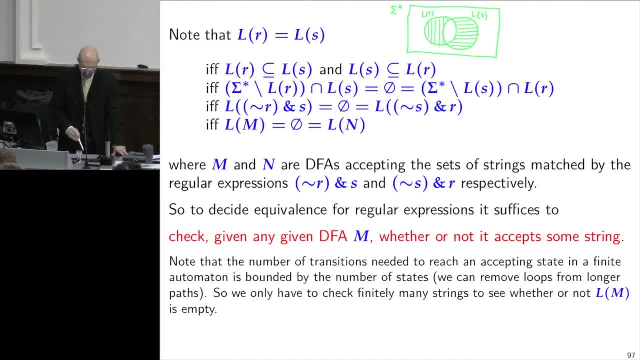 is exactly the same as saying that this part, the whole universe minus language R, would be this area, including the horizontal bars and so on. it's the complement of LR. this is like saying the complement of LR intersected with S. it's obvious when you're thinking about it, if you're explaining to. 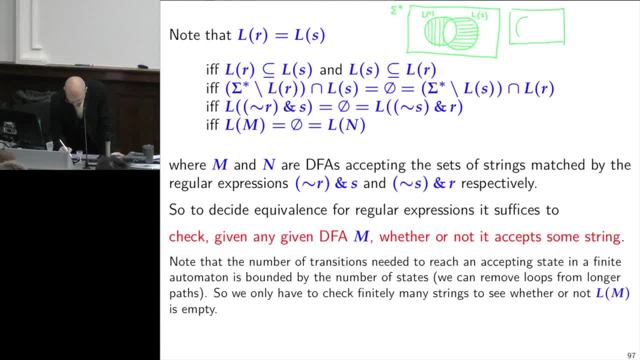 someone who's not thinking about it in their head. you may have to make more drawings. so this first part here is the complement of the first set, so it would be this part, anything that's not in the first set. this part here is this, and therefore their intersection is: 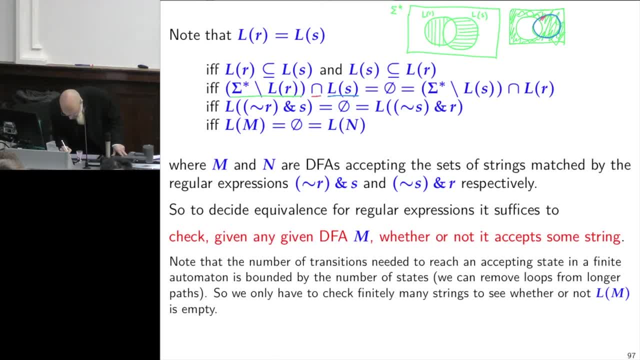 this is the empty set or the thing reversing the sets, and so it comes out the other side and so this is the other one. so if this one is the empty set and also this one is the empty set, that's equivalent to what I said in the. 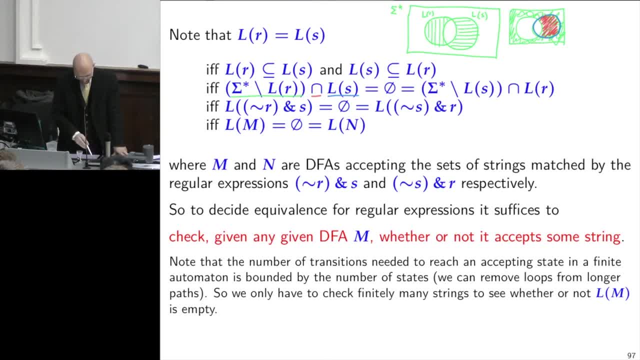 previous slide, or again equivalently, if the language of, not R, which again is the thing that I did in green over here- intersection with S, which is the blue one, and so the intersection is the red one. so that's exactly isomorphic to this, except in the language of regular expressions, as opposed to the language. 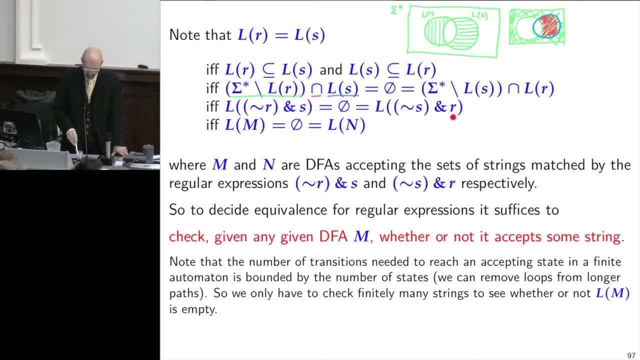 of set theory is the empty set, and similarly on the other side, for this other part, these two things are empty, or equivalently, if the deterministic finite automaton M, which is the one that recognizes the same language as this regular expression, recognizes set of empty strings and so does the one matching this other regular expression. 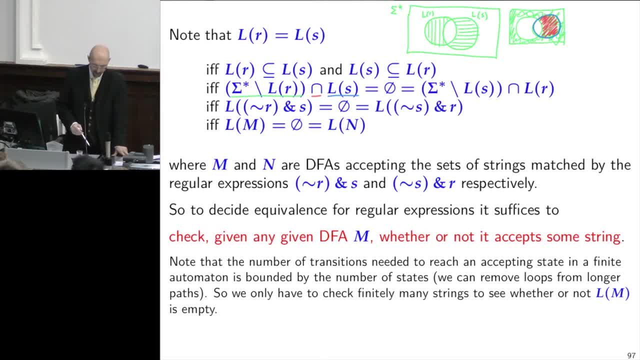 these are all five ways of saying the same thing, and that's when the two regular expressions are equivalent. and so ultimately, if I use my last line, all I need to do- which is actually a lot of work, but the method I may use- is to produce the DFAs for. 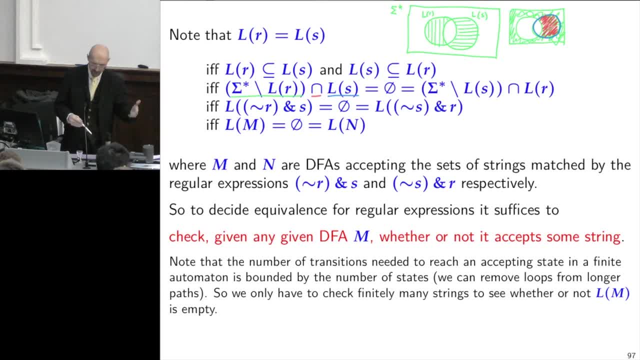 these combined regular expressions. by building up on all the pieces that we built over the past couple of lectures, I know how to make the complement, the intersection and how to make a DFA out of a regular expression. so I do that and that DFA. I need to check if it accepts any strings. 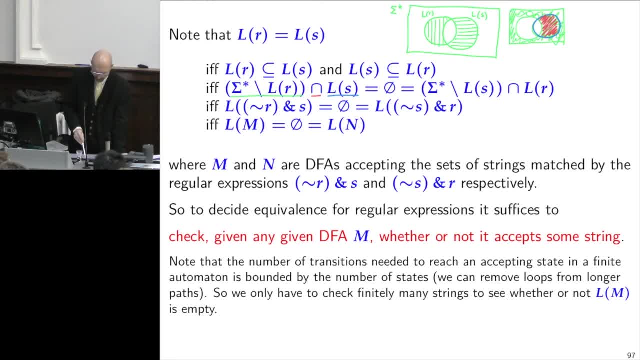 at all. and if it doesn't accept any strings and this other machine also doesn't accept any strings, then I'm home. how do I check if an DFA does not accept any strings? there are some DFA that you look at them and it's obvious that they don't accept any strings, for example, because they don't 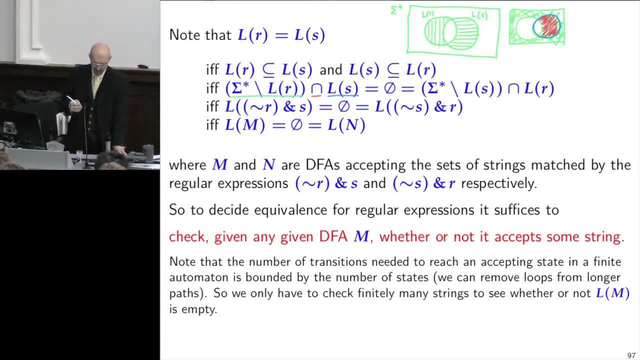 have any accepting states. but that's in one direction. we actually in the other direction. if I look at an arbitrary DFA, how can I establish whether it is the case or not that it doesn't accept any strings? and it may well have a certain state, except that no string reaches the accepting states, and so you. 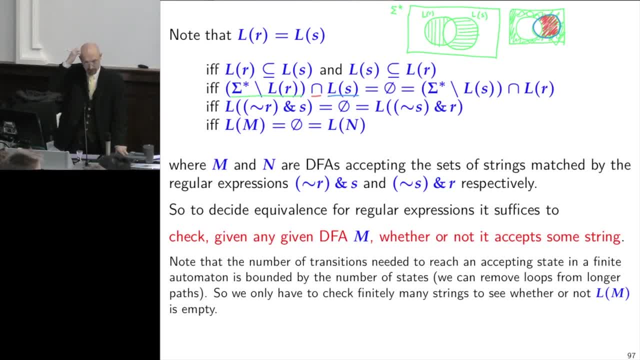 have to actually check more carefully and just seeing if there are any. acceptance is the interesting thing is because a DFA by definition has a finite number of states, from the starting state to any of the accepting states. there's only a finite number of possible paths and so the number of things you have to